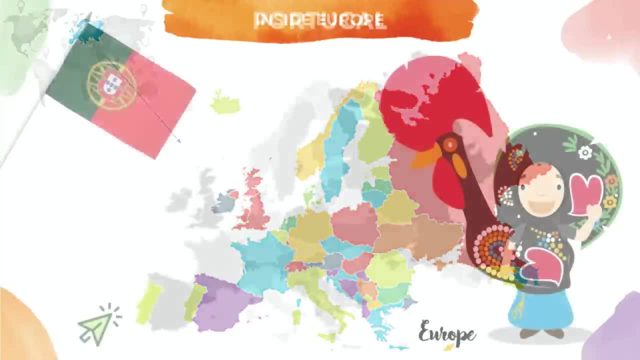 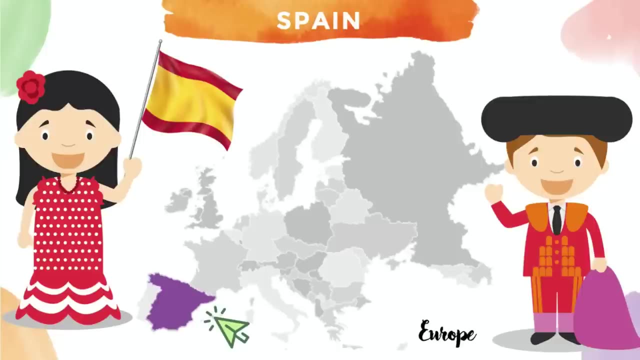 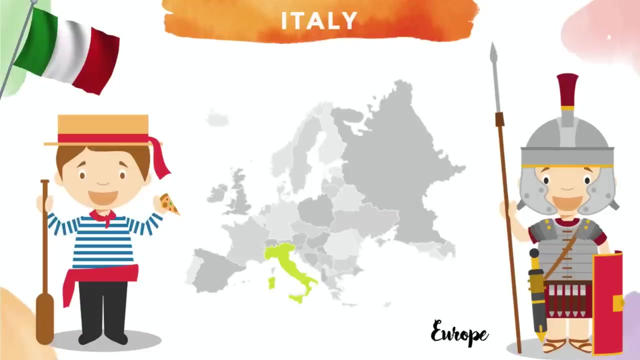 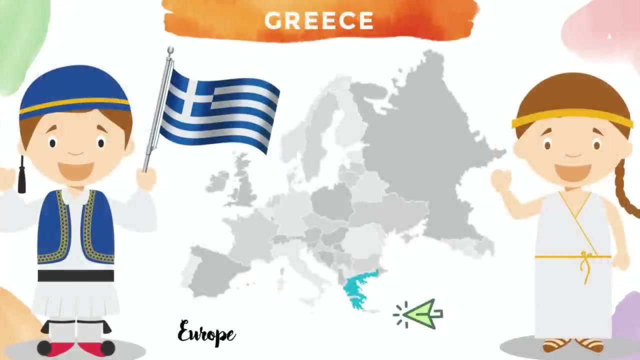 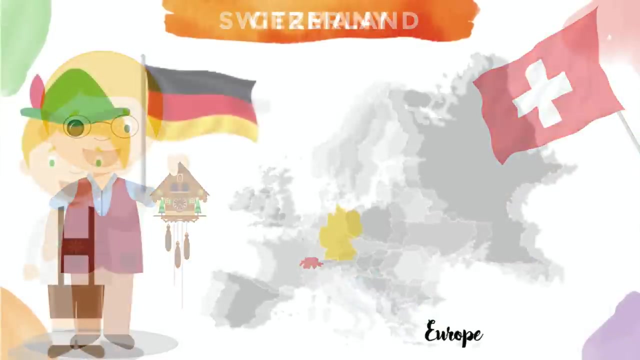 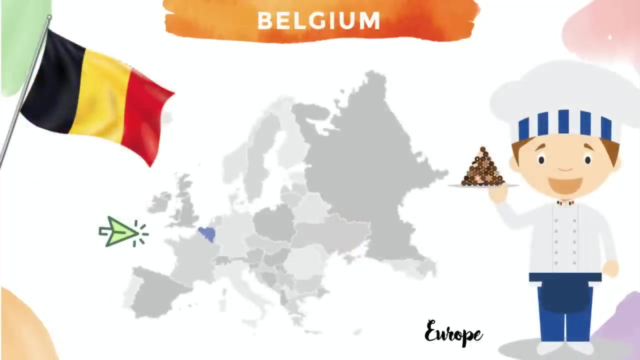 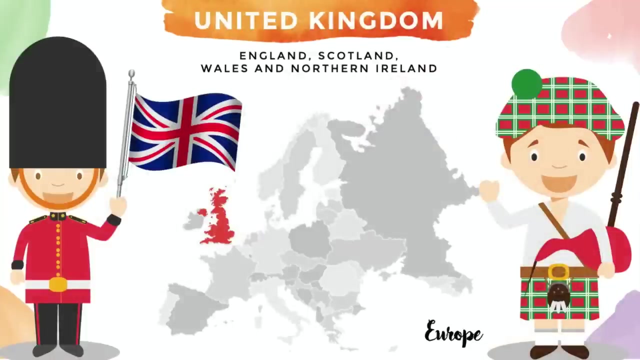 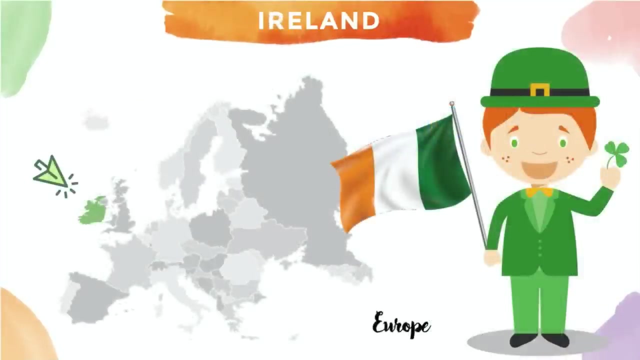 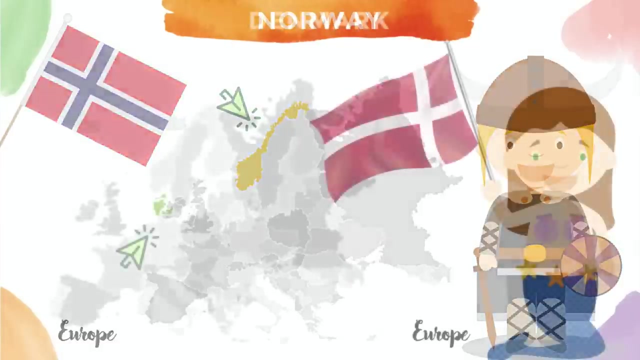 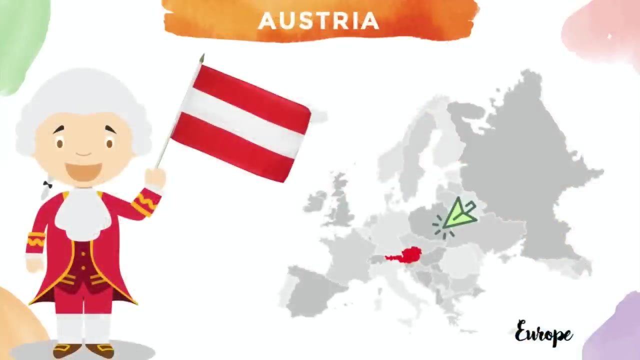 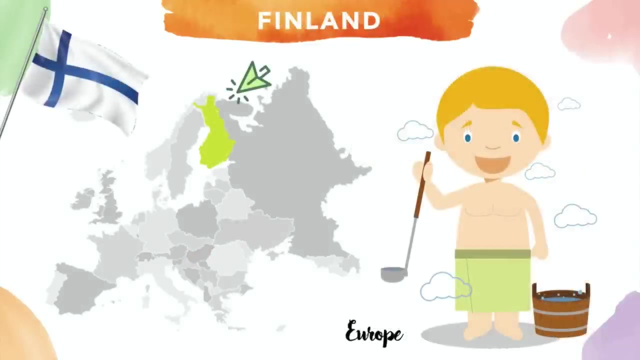 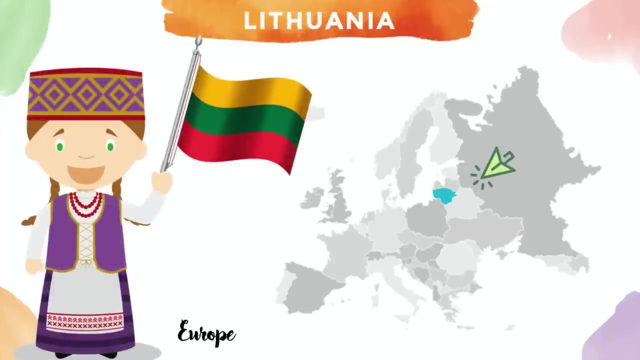 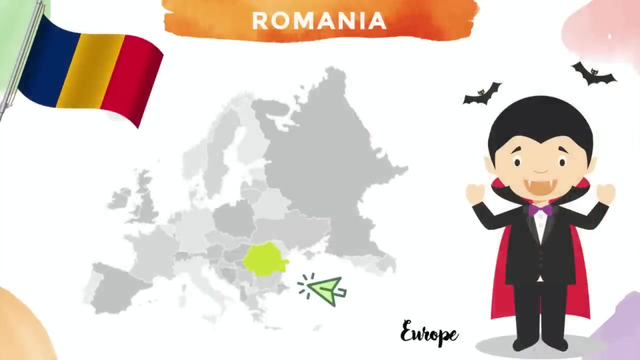 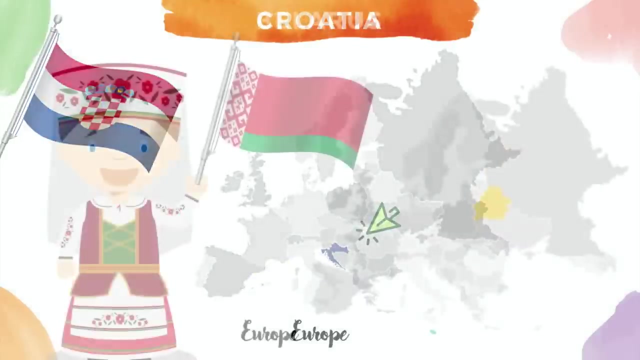 Inside Europe we can find Portugal, Spain, France, Italy, Vatican City, Greece, Switzerland, Germany, Belgium, Netherlands, United Kingdom, Iceland, Ireland, Norway, Denmark, Austria, Hungary, Finland, Lithuania, Bulgaria, Romania, Croatia. 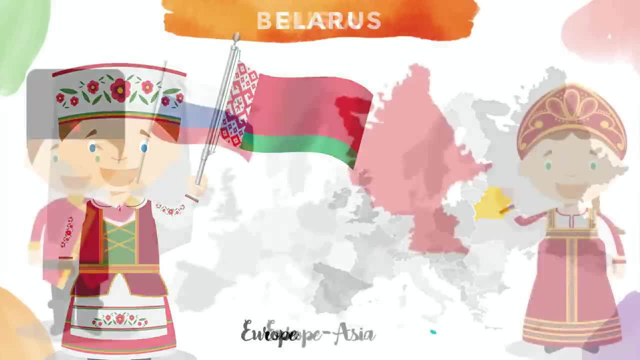 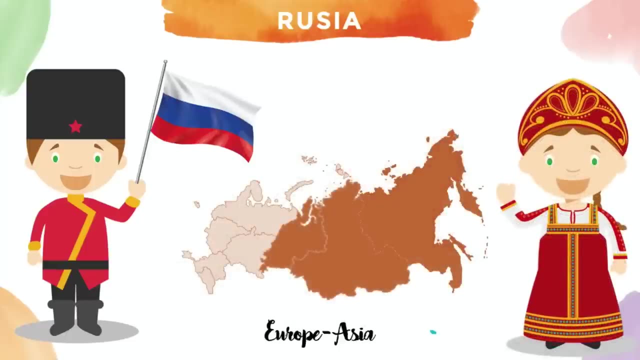 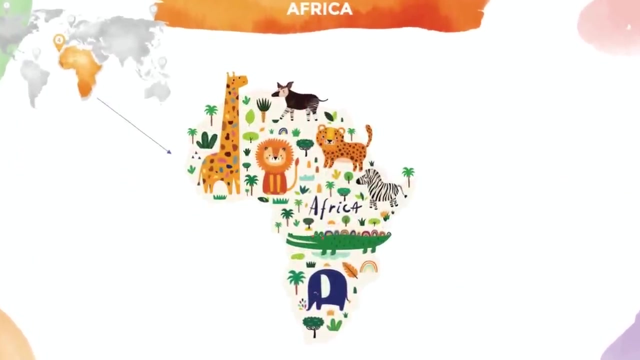 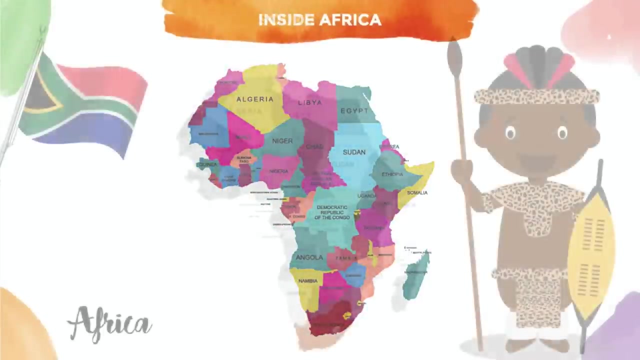 Belarus, Russia. Russia is part of Europe and Asia Also Turkey part of Europe and part of Asia. Next continent is Africa, where you can find many exotic animals. African countries are South Africa, Egypt, Morocco, Algeria and Africa.